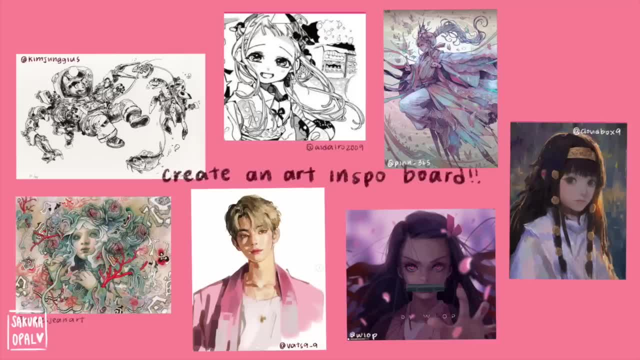 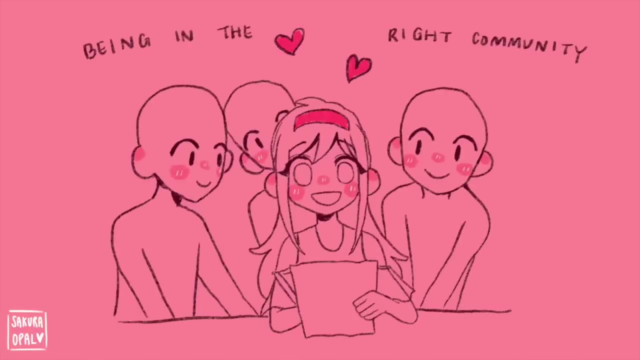 are actually amazing. If you're interested in learning more about art, please subscribe to my channel and hit the bell icon so you don't miss any of my new videos. I'll see you in the next video. Step two is being in the right community, because that can really encourage you, and especially as a 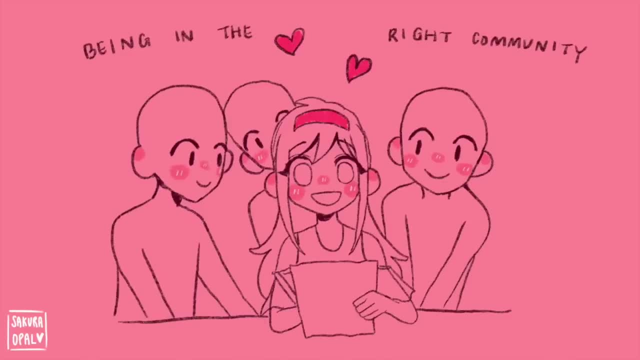 beginner artist. a lot of them don't have the confidence, which is totally fine because it's something that comes with time. but having fellow artist friends to support you will make you feel safe and obviously it'll be really fun because then you guys can do art, trades, collabs, etc. 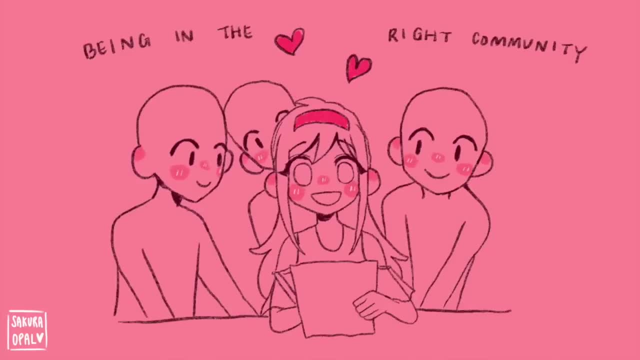 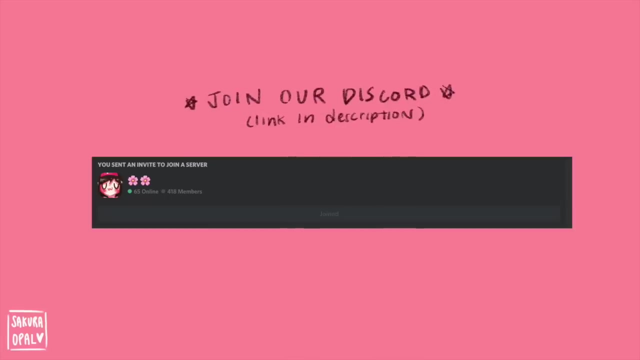 When I first started I didn't really have an art community that I think I belong to, but after I found fellow artist friends and a community like the one I have now, that really pushed me to draw more, and this is a shameless promo, but we have a small wholesome Discord community here, if you. 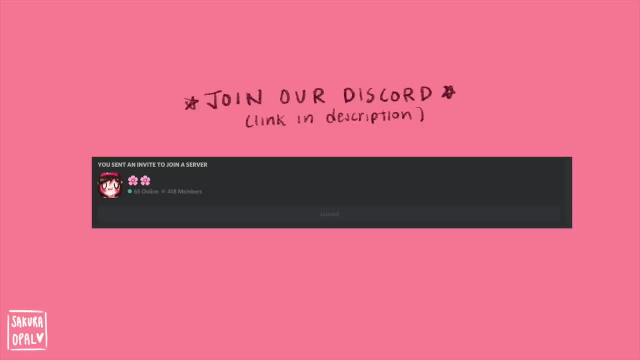 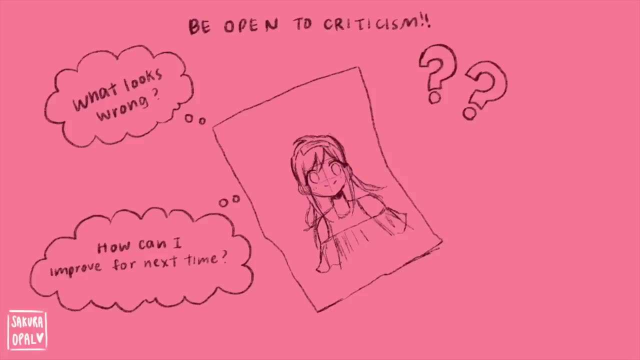 want to share your art too, if you don't have one, I think it'd be really cool if you joined. Yeah, Step three is to always, always be open to criticism and ask people for advice, especially if you think something looks off but don't know what, because that happens a lot in art and after 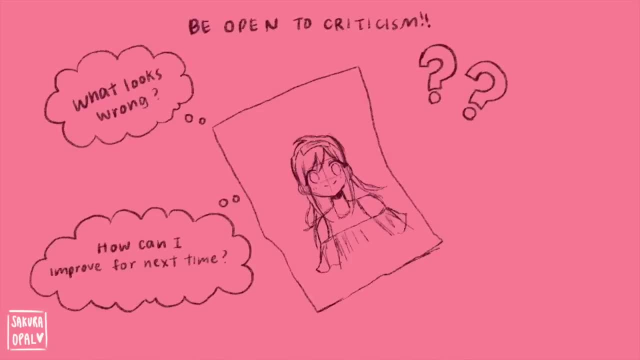 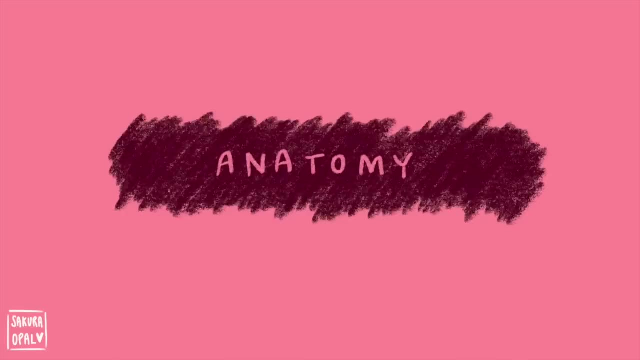 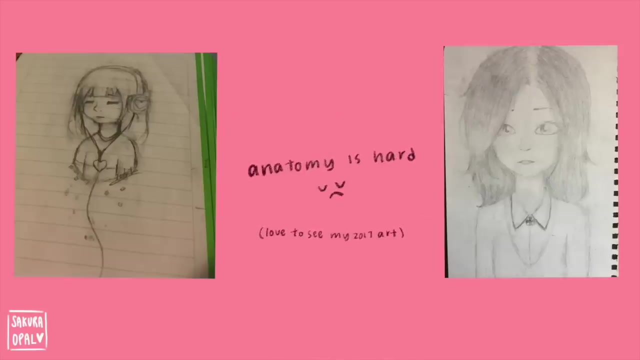 you figure out what looks wrong. remember to make a mental note and then fix it in your next drawing. I used to struggle so much with anatomy too, and I always stuck with headshots and stuff because of it, but that isn't what you should do, because you'll never improve if you 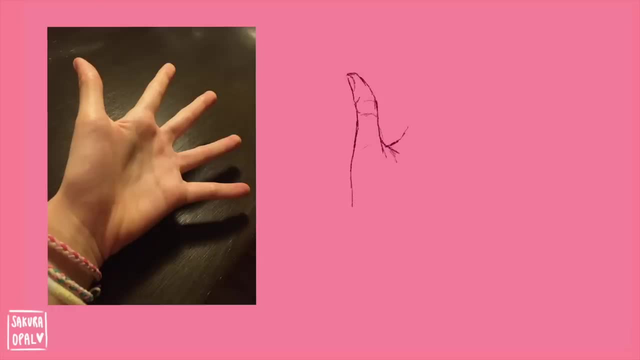 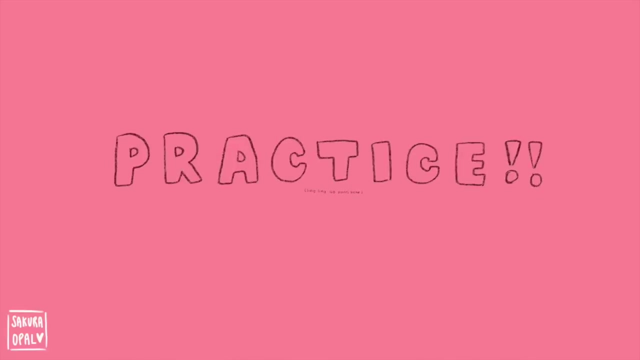 never draw bodies, So one tip I will give is to use a lot of references, Just google images, use the mirror or just take pictures of yourself as a guide, and especially for the hands, because that can be really hard and it's a lot of practice. so it takes a long, long long. 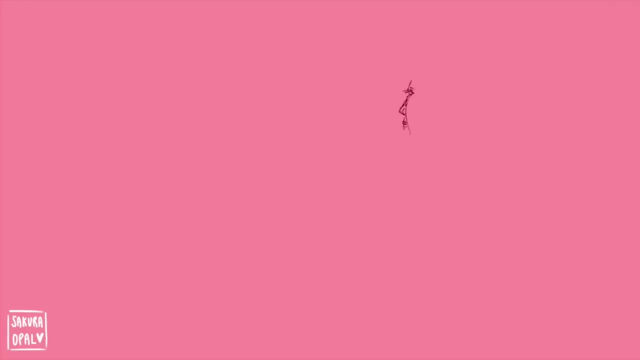 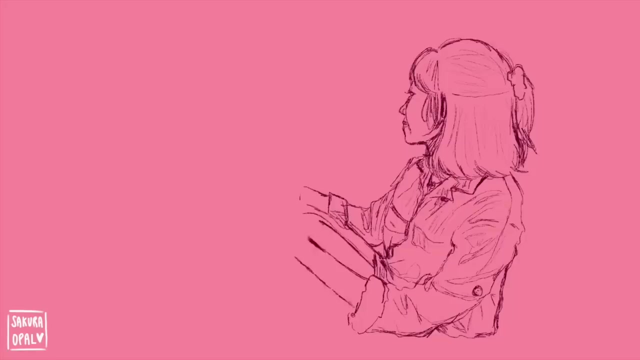 time to get the hang of anatomy. and also another tip I would give is to practice drawing life figures. Obviously you don't have to draw nude figures- it can be figures with clothes on- but just looking at the form and shapes and just drawing a lot, then your anatomy will. 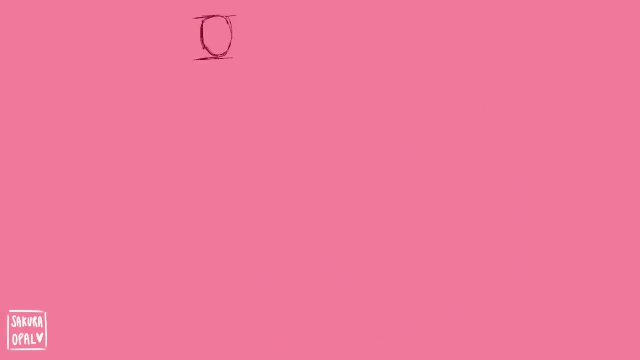 improve, improve along with it. One more thing that I would like to give you guys is that there is like an average height dimension thing. so an average adult woman around seven and a half heads tall. so as you can see here, it's split up to seven heads, like the. 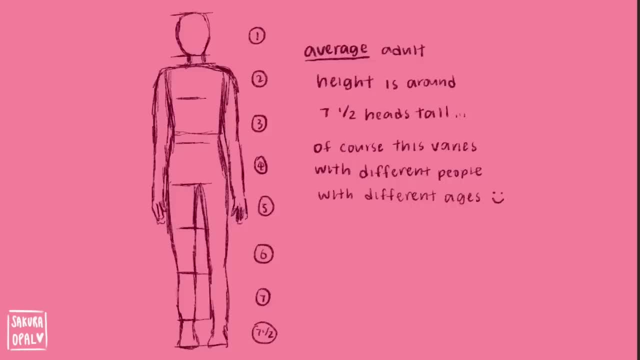 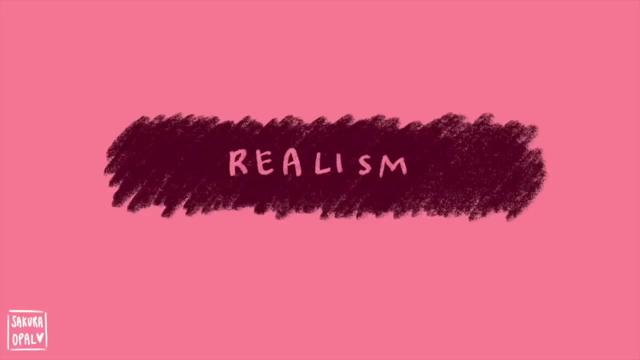 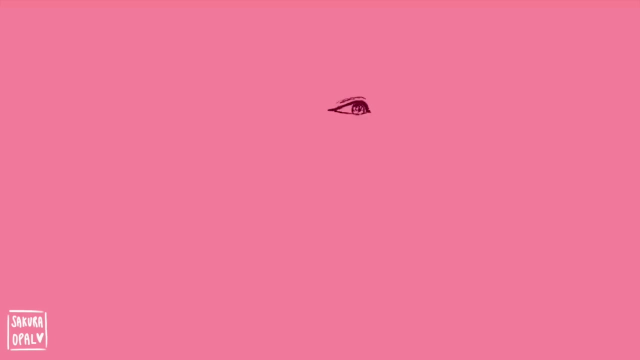 length of seven heads plus one half of a head, and then obviously this varies with different people, but here is just a small guide to keep in mind. So some of you guys asked me how to do semi-realistic or realistic drawings, but honestly, I would just tell everyone that I don't know how to do realistic or semi-realistic drawings. 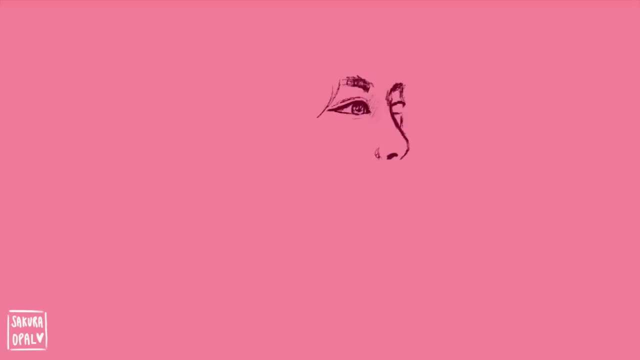 Everyone to start doing realistic right now, whether you like it or not, whether if you only want to draw anime or not, because this will tremendously improve your art, and I cannot stress on this enough. So now you may be wondering why I'm making everyone do realistic. because if 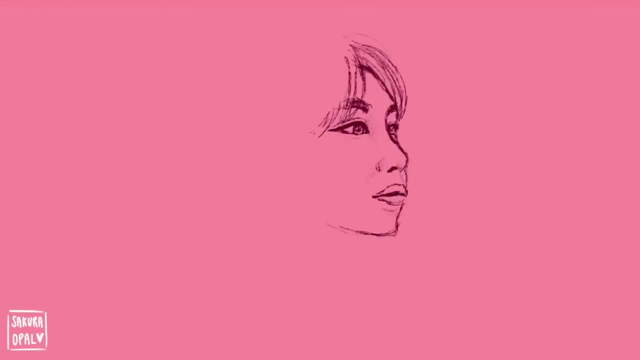 you think about it, everything is based on the real world, so even anime is based on the real world. so it's important that we know how to draw the real world first before we draw anime, if that makes sense. and if I could give one piece of advice to my past 11 year old, 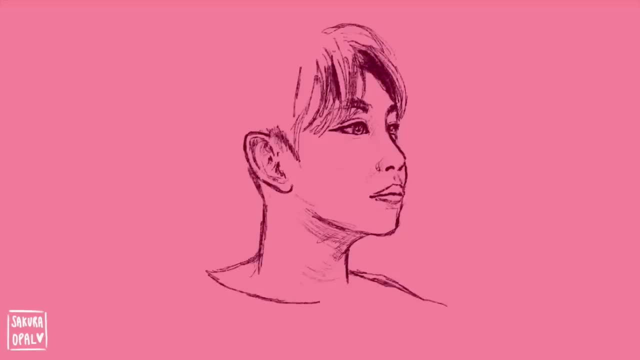 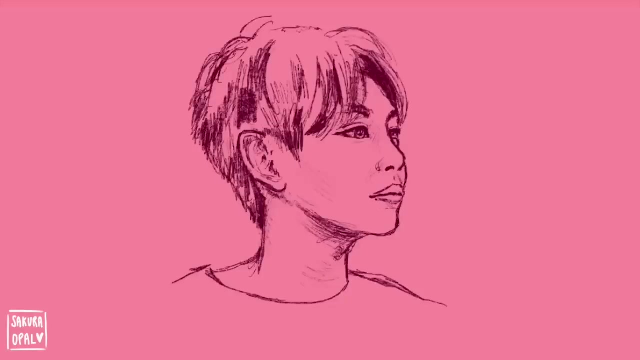 self this would be. it is just to draw a lot of realistic art. Obviously, you can still draw anime, but just make sure you have a balance between the two and you are practicing realistic as well. and how to start practicing for realistic is to do a lot of studies. You can just take photos, find photos. 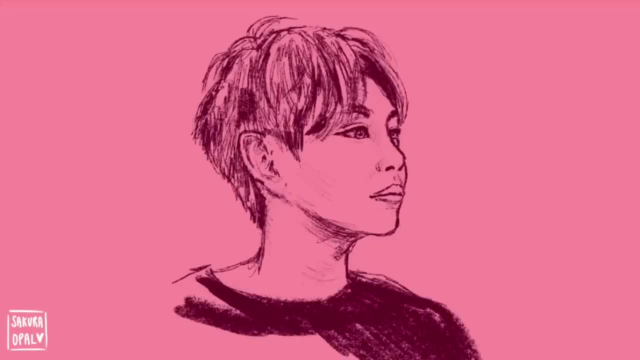 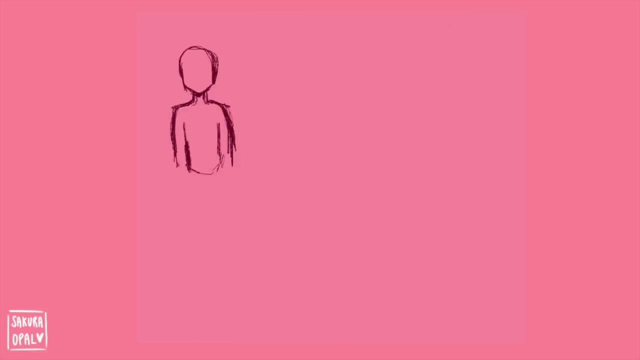 or just draw what's in front of you in real life and instead of looking at like the symbol, you will look at the shape and form, and that will really help you draw well. Another advice I would give is to when you're drawing, especially digitally, it's really easy for you to flip the canvas. 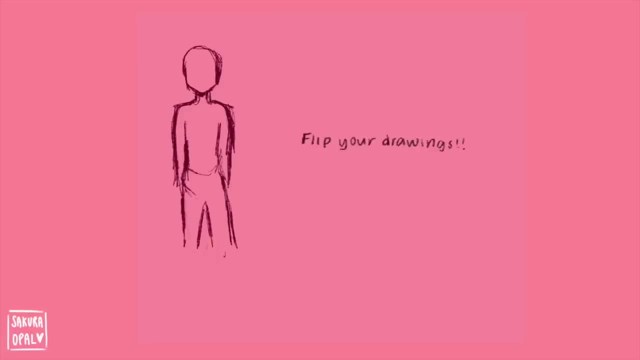 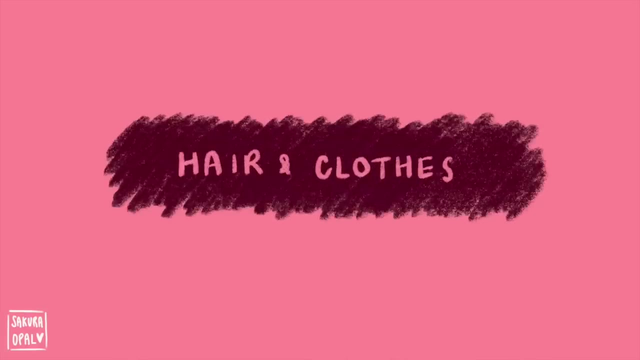 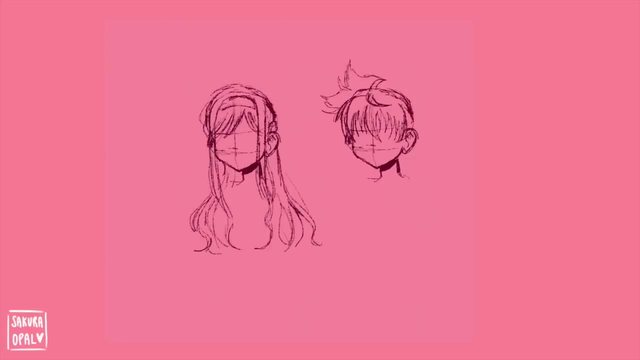 horizontally so you can see what looks off, and I always use that to see figure out what looks off in my drawings as well. For hair, the number one advice I would give is to think of it as sections or blocks, instead of thinking of it per strand. 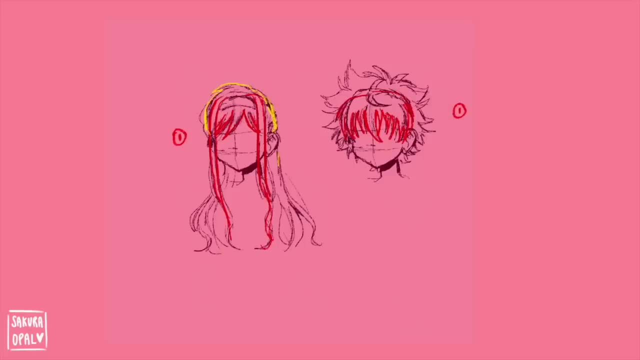 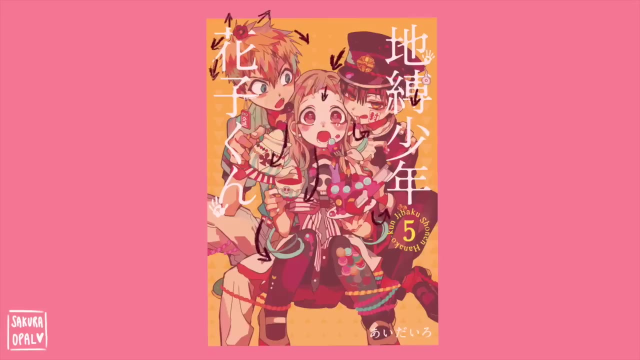 So, as you can see in the example here, the red would be one section, the yellow would be one section and then the green would be one section. and also one thing to keep in mind is the direction of the hair. So if it's short hair, like you see here, it would go in different directions, like around the. 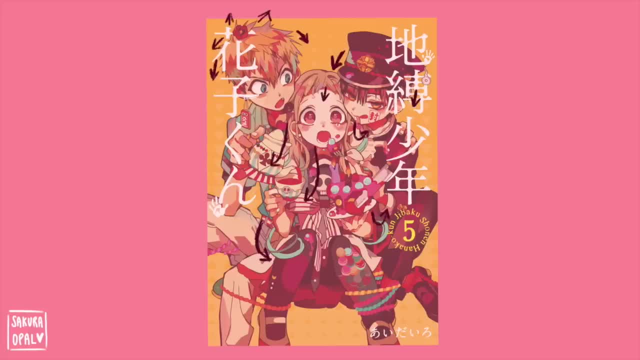 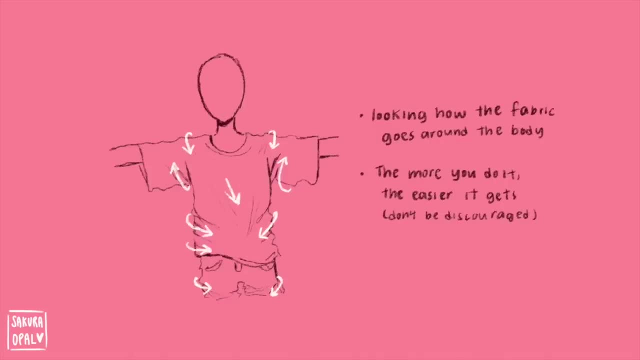 the scalp and if it's like long hair, then it usually would flow down because of gravity, if that makes sense. And as for clothes is to think about how the fabric goes around the body, and this is something that a lot of. when I was a beginner artist, I really did not know how the 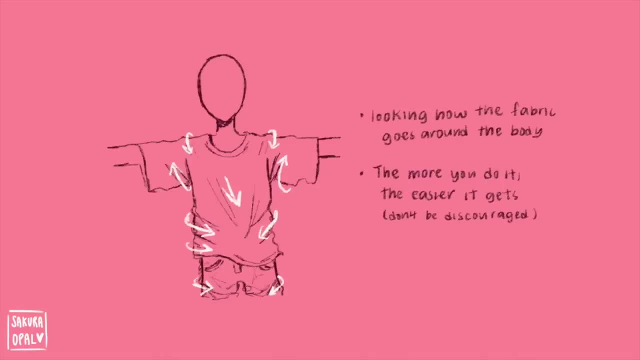 clothes folds work. So it really comes with time and the more you do it, the easier it gets. and, as I said before, if you don't know how to fold your clothes, you don't know how to do it. So it really comes with time and the more you do it, the easier it gets. and, as I said before, if 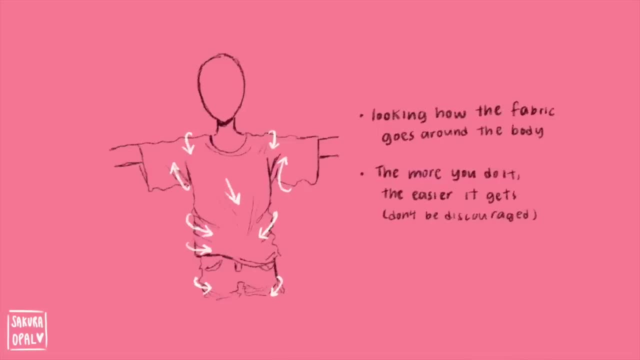 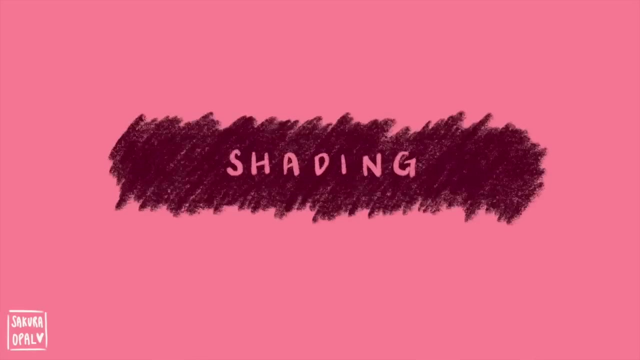 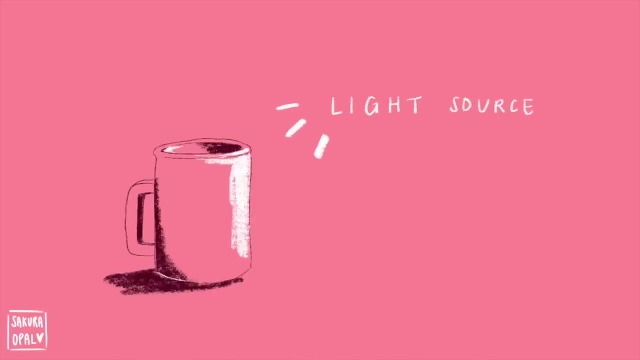 you do more studies, then you'll probably be able to pick this up quicker. so yeah, For shading, the key point is knowing where the light source is, so then afterwards you can determine where the shadow and the highlights will be. So, as you can see here the closest point. 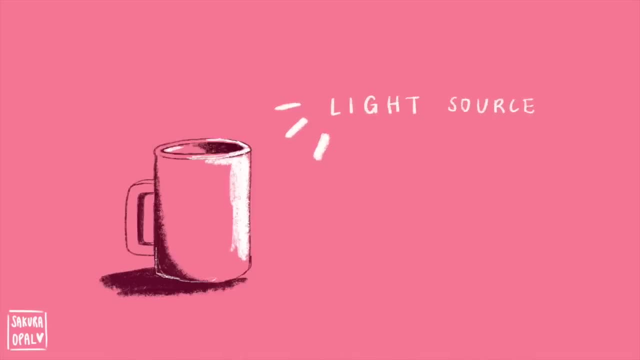 from the mug to the light source will be where the highlight is, and then the shadow will be in the opposite direction, And then the light- the direction of light- will cast the shadow in one direction. so please keep that in mind, And here is also some examples of where the shadows and the highlights would be if the light source is in a different location. 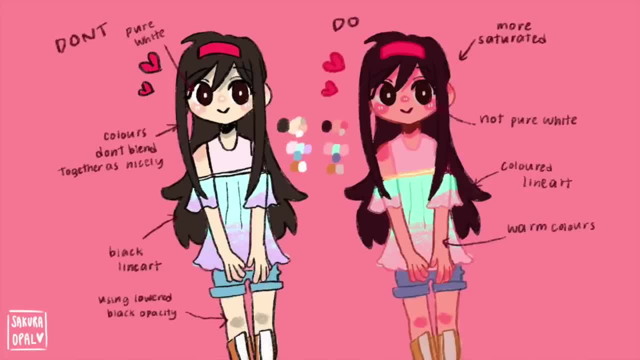 For me. I think color is one thing that took a lot of time and experimentation and it definitely won't come after finishing my work. I think color is one thing that took a lot of time and experimentation and it definitely won't come after finishing my work. 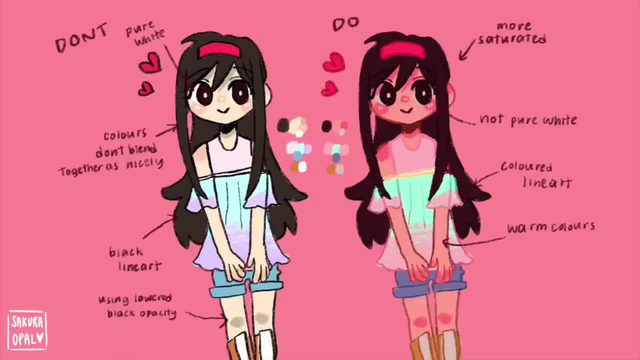 I think color is one thing that took a lot of time and experimentation and it definitely won't come after finishing my work is when you get to the drawing part, is when I was finishing two drawings and it takes, as I said, a lot of time. so I personally like a lot more saturated colours because for me that really makes my 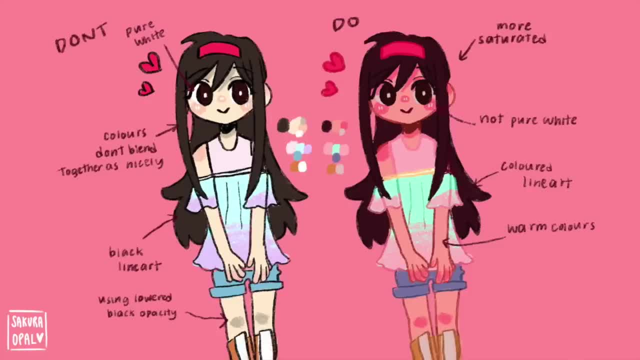 artwork pop out and stand out more and you can see here in the comparison to a duller colour scheme on what to do. and one thing is to not have black as your lineart and usually coloring your line art will also make your drawing stand out a lot more and also just. 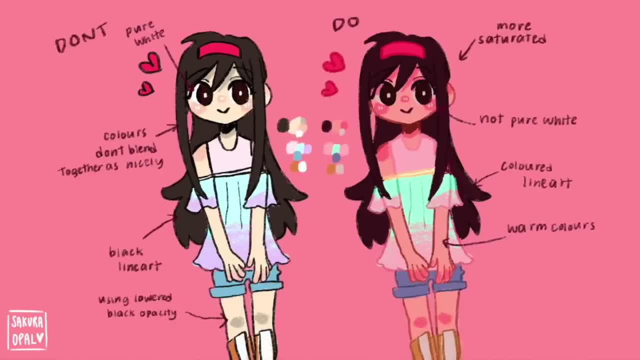 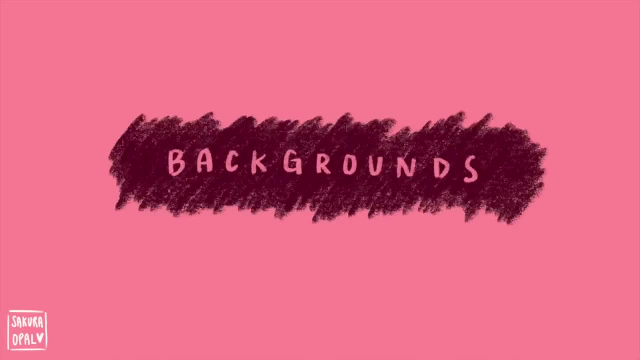 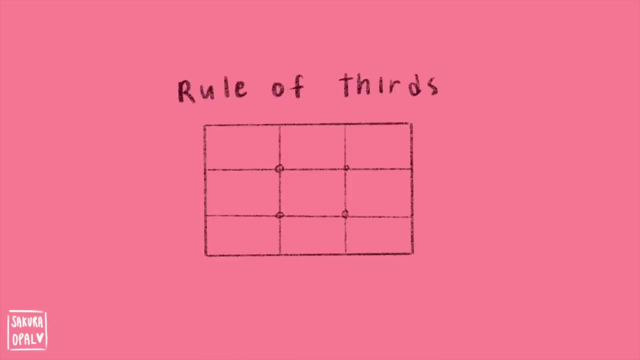 just having determining if your palette is warm or cold. that can also really affect the overall mood of your artwork. For backgrounds, there are four key concepts that I keep in mind when creating mine. so the first is rule of thirds. if you don't know, it's a rule that, if you, you should generally put. 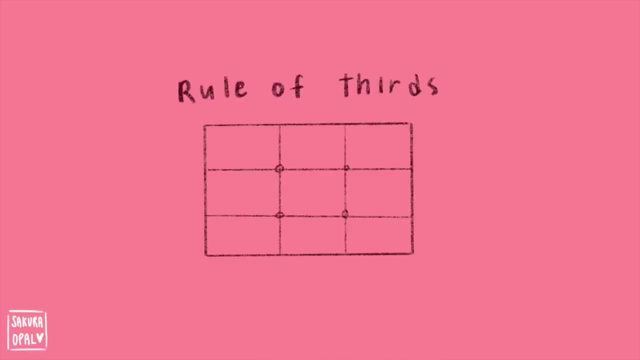 your subject close to the lines, especially the intersection points of the rule of thirds, as you can see on the small chart that I did. The second thing is to know where the vanishing point is when creating the background. so imagine you're looking out on a long road. you probably can't see the end. 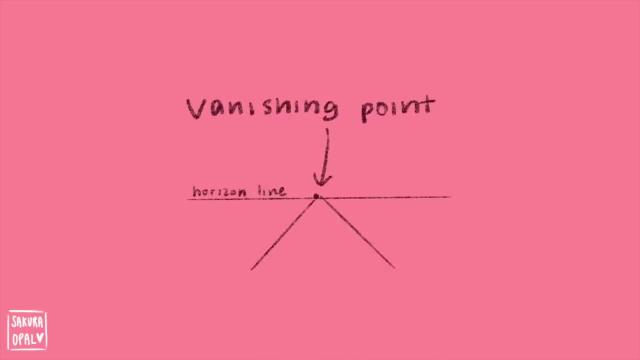 and the furthest point you can see is the vanishing point, and then you can see the objects going closer towards. the thing is getting smaller. so that is also something to keep in mind. the third is to have consistent lighting, so that will really make the subject really blend in. 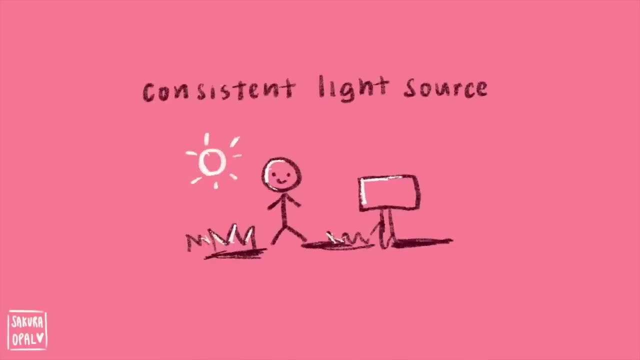 with the background more and so, as I said in the shading is to know where the light source is hitting the object from, so you can determine the shadows and the highlights. and four is color schemes. so making sure you can either use this in two ways: making sure that 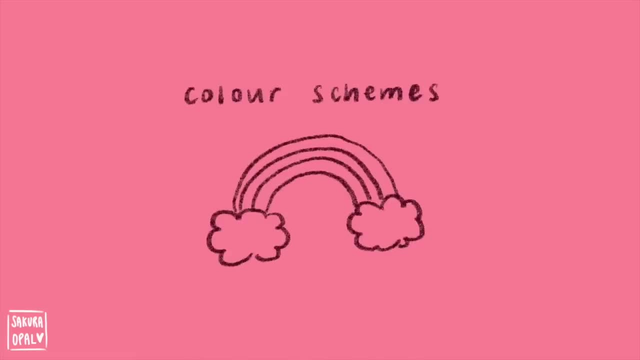 the subject blends in with the background and�� Peninsula auxıyla the object is hidden as well as the lighting of the background. isən pourquoi Pennsylvania, auxiliavielThanbildja negvolda blends in, or if you want the character to stand out, then you would use a contrasting color scheme. 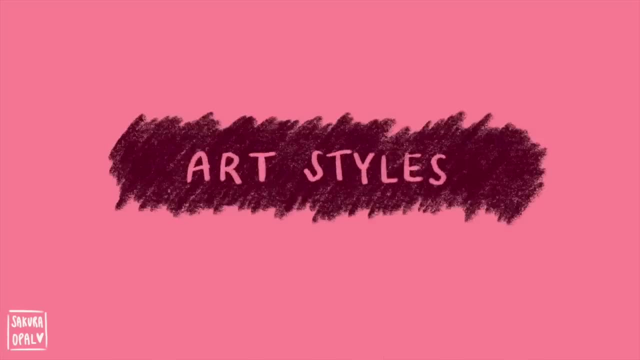 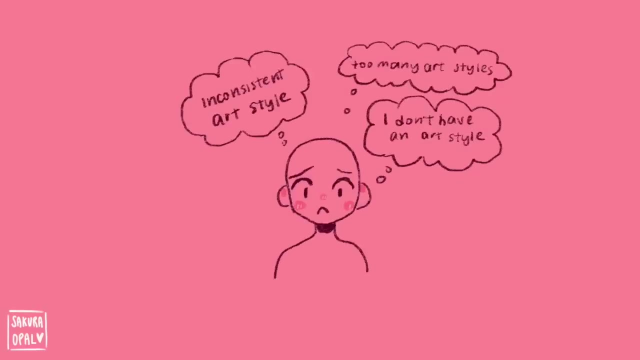 a lot of beginners complain that they don't have an art style or they don't have a consistent art style or they have too many art styles. but i don't think these are necessarily bad things, because if you have multiple art styles, that just shows that you're willing to experiment. 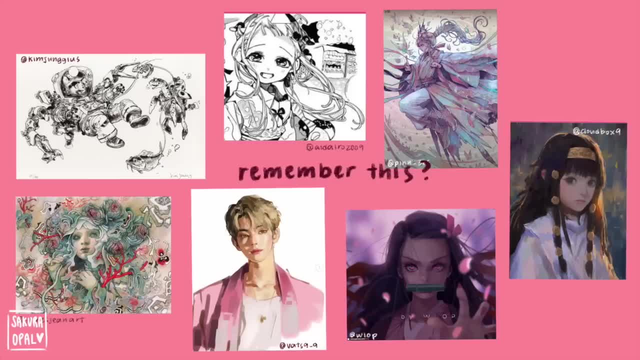 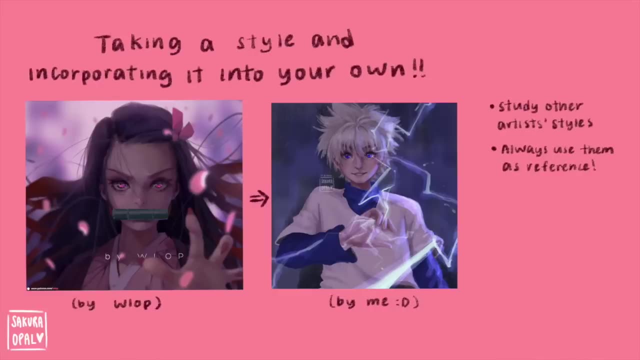 and you're willing to try something new. so remember the art inspiration board from earlier. so then, what you do is that you take artists that you really admire and put their try to incorporate their art style into your own art. so you can see, here is an example, one of the artists. 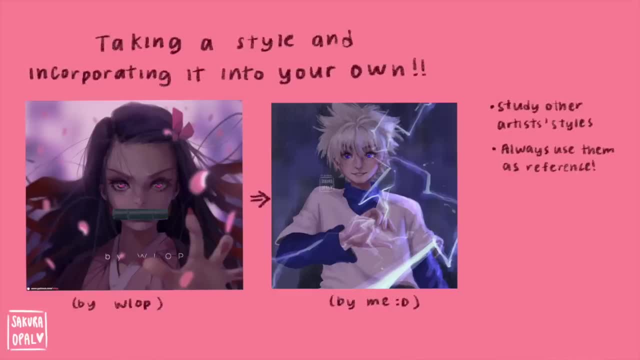 that i really like volop. i don't know how to pronounce, i'm sorry if i'm pronouncing it wrong. um, i would take their art style and then i would just incorporate to my own version, so you can see. then i created this new art style and you would always use them as a reference. 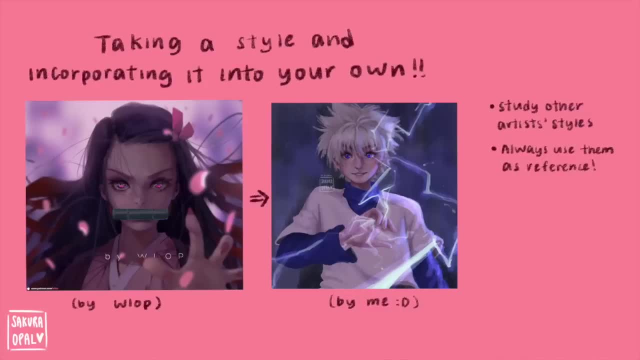 so that's why i said earlier that you should be able to access this art inspiration board really easily, so you can always go back to it. and another thing is that you can take multiple artists and incorporate it to your own art. so, for example, i like how this artist draw eyes. 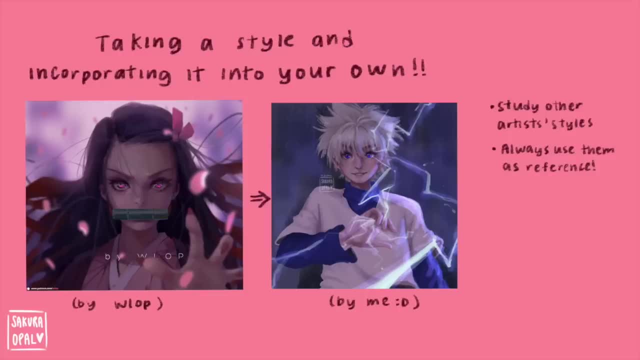 so i put that in my art. i like how this artist colors. i would put that in my art and it's just. you can see that i've created this new art style and you would always use them as a reference. your art style would become the amalgamated form of all these art styles combined. 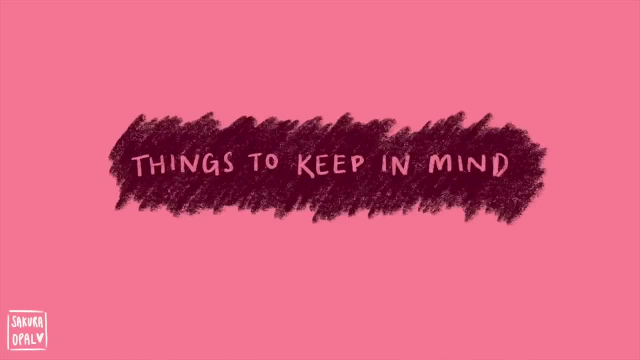 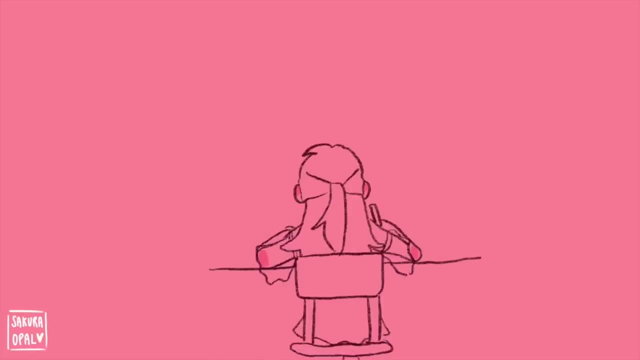 these are just the things that i think an artist should know when they are starting to draw. so the first thing is to know that you should be in the zone while you're drawing, because that will really make your ideas flow out more, and you'll know when you're in the zone is when you aren't really. 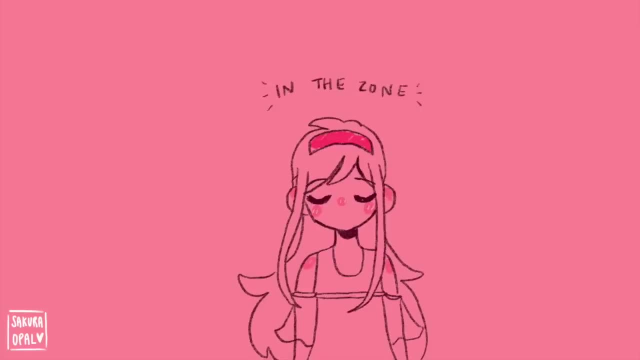 distracted and you lose sense of time, and that also means that you're using the more visual side of your brain, if i go into the psychology of things, and that is the side you're supposed to be using while you're drawing. so that means you're doing a good job. and one thing for me: 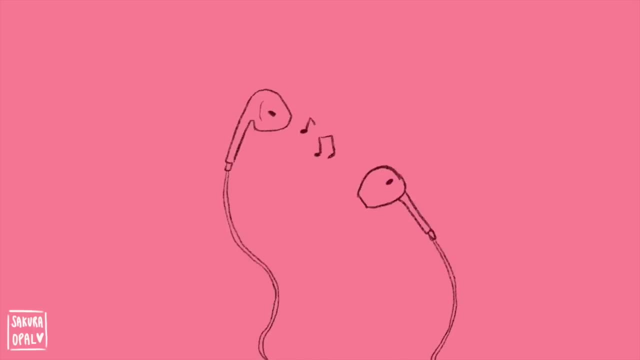 to get into this zone is to listen to music. so it's okay to listen to music when you're drawing or listening to anything for me, but it can be anything for you, and that's it for this video. i hope you enjoyed it and i'll see you in the next video. 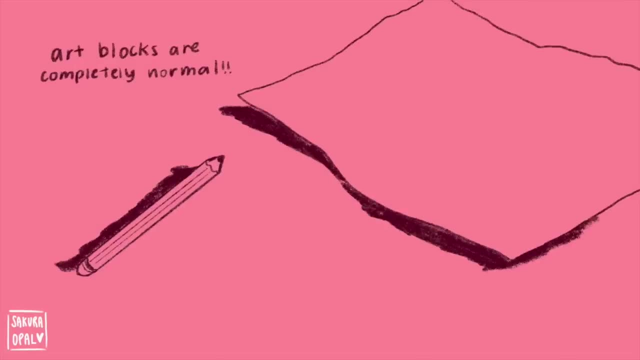 another thing i wanted to say is that art blocks are really normal. so please don't be frustrated if you have an art block. so if you have an art block, things i would do is to remind yourself why you like drawing and just take breaks- and it's okay to take breaks and also have a good mindset that. 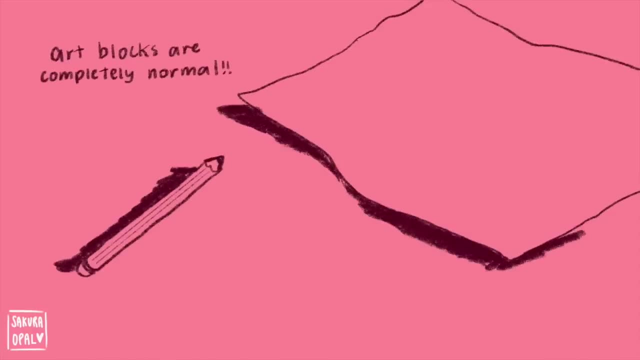 you'll improve with time and it'll take time and practice, like all other things. so that's all for this video. i hope you enjoyed it and i'll see you in the next video. thank you for this video. i hope this video helps in any way and if you ever have any questions, feel. 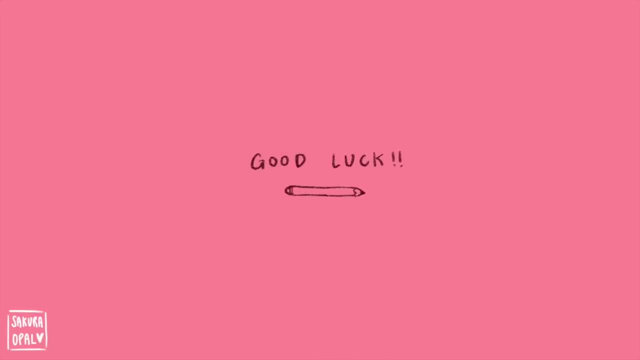 free to dm me, or you can ask me for art critiques, because i love helping younger artists improve their art as well. so yeah, that's all, and see you guys in the next video.